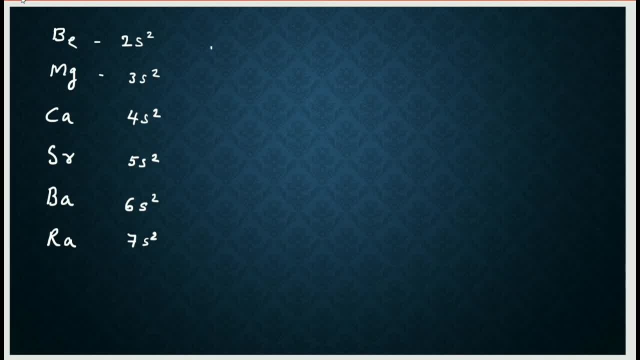 down the group, the size increases. So down, the group size increases, always Size increases. And when we discuss group 1 element, lithium sodium, the outer electronic configuration was for lithium it was 2s1, for sodium 3s1 and so on. So in group 2, elements, the size. 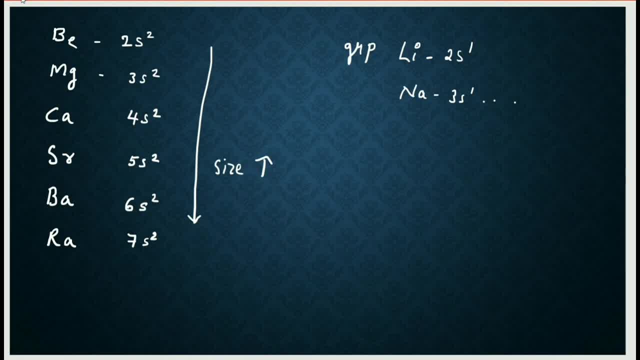 increases down the group, similarly like group 1 elements. and what about the ionization enthalpy? Ionization enthalpy is proportional to 1 by size. That means size increases, ionization enthalpy increases. So beryllium having 2s2 configuration, removing one of the electron from 2s orbital is difficult. 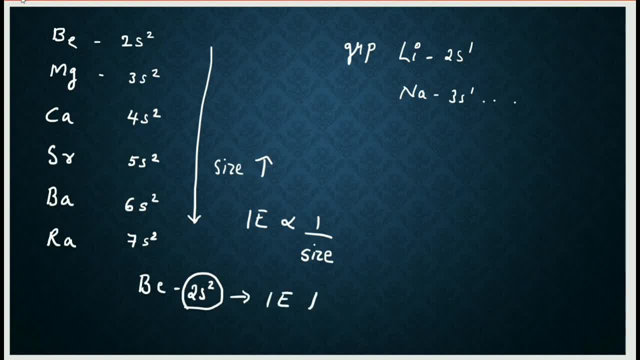 That means ionization enthalpy is greater. We need more energy to remove one of the electron from 2s2 subshell, So ionization enthalpy is greater for beryllium, Since size is small- size small, ionization enthalpy greater. So ionization enthalpy order. 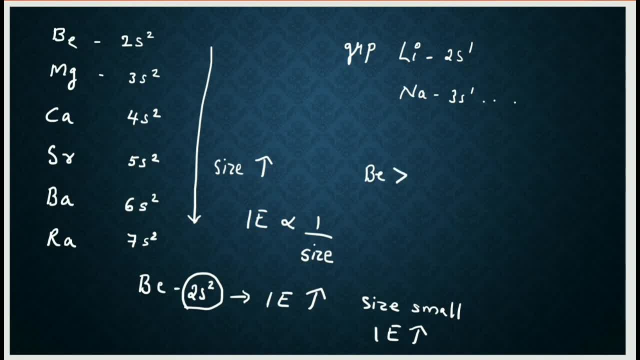 is beryllium having greater ionization enthalpy, then magnesium, then calcium, then strontium and barium. And what about the second ionization enthalpy? When first, ionization enthalpy means to remove the first electron from the outermost ship. Once one electron has been removed, 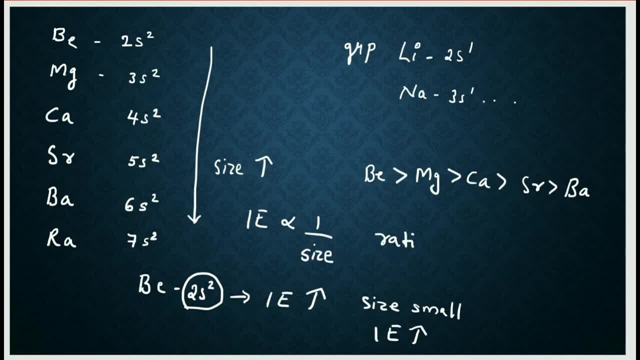 the ratio of charge of nucleus to orbital, ratio of charge of nucleus to orbit. Nucleus to orbit will be greater, So nucleus to orbital will be greater, So the electron will be strongly held by the orbit. So electron is strongly held means it is difficult to remove this electron from the orbit. 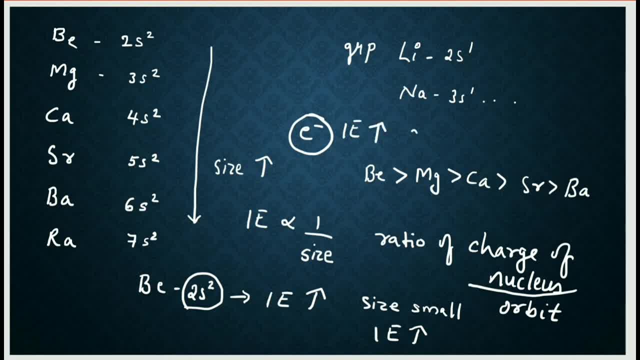 So ionization enthalpy will be greater. that means, second, ionization enthalpy is higher for group 2 element compared to group 1 element and size of the group 2 element is small compared to group 1 element means ionization enthalpy will always larger for group 2 elements. 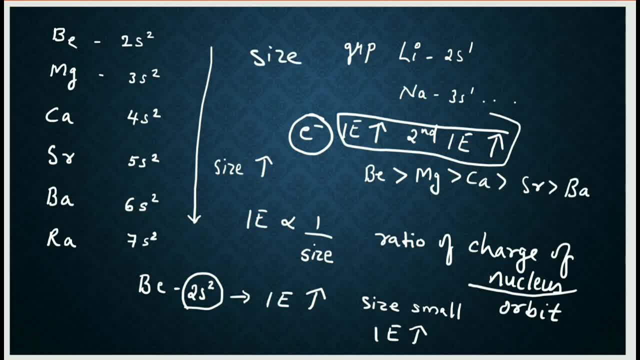 So size: small size is small compared to group 1 element. group 1 element and ionization enthalpy: ionization enthalpy is larger for group 2 elements. So just remember: size, small Size, small, ionization enthalpy greater. size is small, ionization enthalpy greater. so that's about. 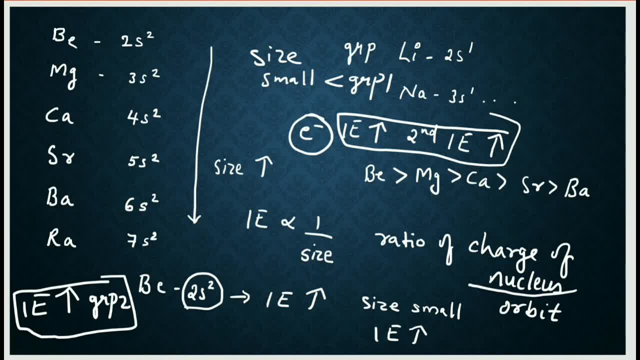 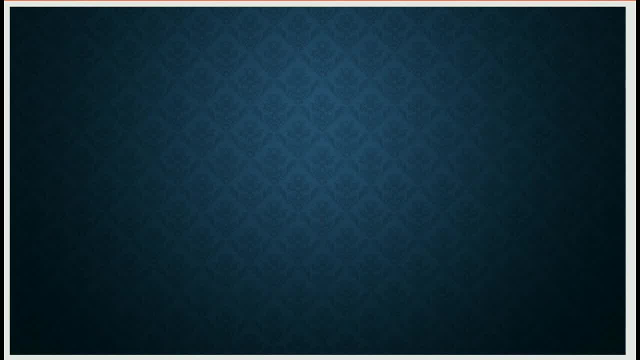 ionization enthalpy order. Now moving to electronegativity. so these are metals, these are electropositive elements. so alkaline earth metals and alkali metals are electropositive. electropositive positivity is greater. electropositive is greater. that means 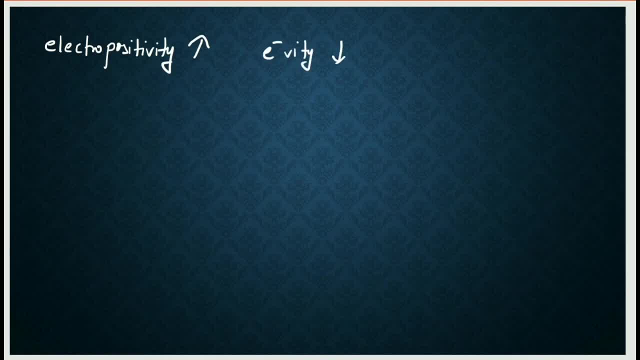 electronegativity. The electronegativity value is low for alkaline earth metals, so lower electronegativity values, but compared to group 1 elements it has high value. when comparing group 1 elements, group 2 have high electronegativity than group 1, so generally low electronegativity value, but group 2 have 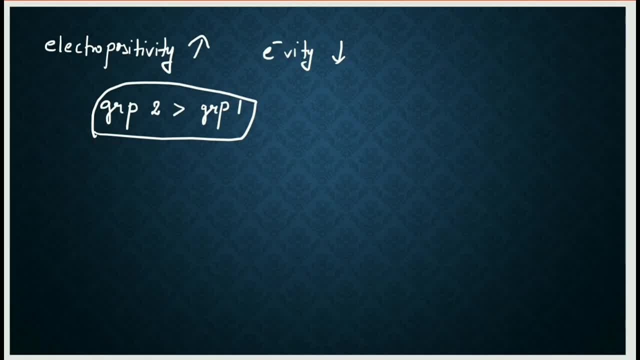 high electronegativity value compared to group 1 atoms. Now hydration energy. so hydration, when talking about hydration energy, four or five times greater than group 1 ions. so four or five times greater than greater than group 1 elements. so group 2 elements have high hydration energy compared to group 1 elements and hydration energy decreases. 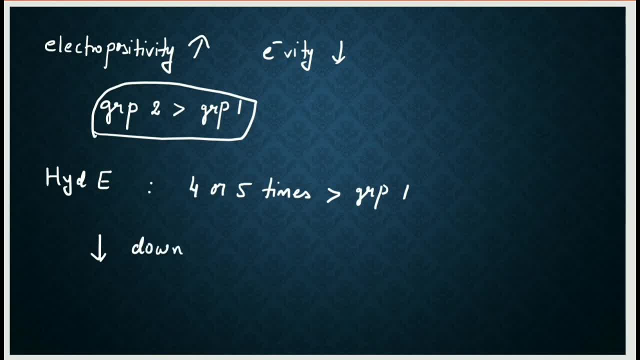 down the group. when you move from down the group, So the size increases and hydration energy decreases. so hydration energy decreases when you move from top to bottom of the group. so that's about hydration energy. Next one is what solubility? so solubility is depending upon the atomic weight. the atomic weight increases and the solubility decreases. 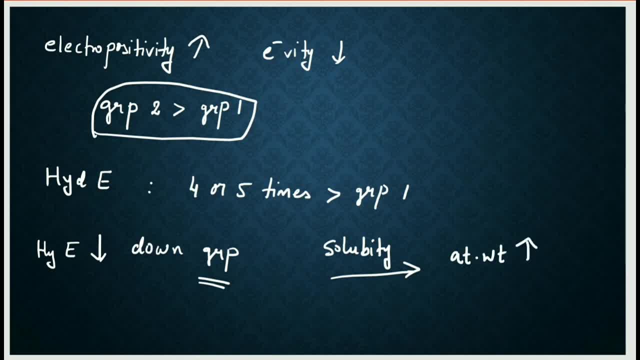 atomic weight increases, solubility decreases. So atomic weight increases, solubility decreases means beryllium, magnesium, calcium, So, which is having higher atomic weight. Calcium is having higher atomic weight, So solubility will be low for calcium. Solubility will be low for calcium. 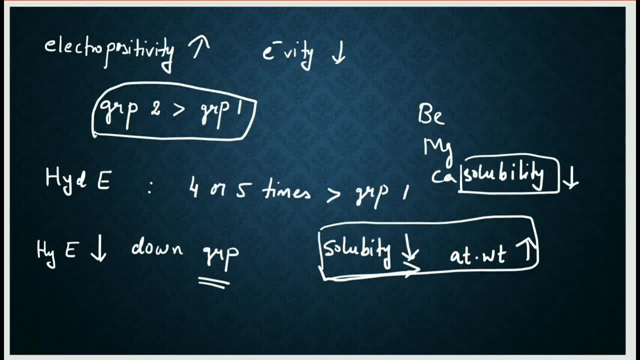 salt and there is an exceptional case for solubility. also the fluorides and hydroxides. fluoride and hydroxides have reverse order. that means for calcium salts- all other calcium salts- the solubility is low. but when coming to calcium fluoride or calcium hydroxide the solubility is. 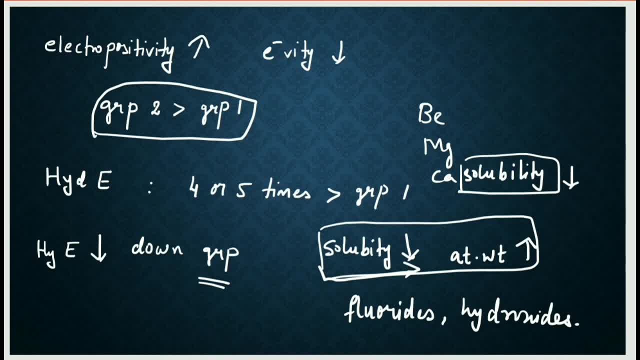 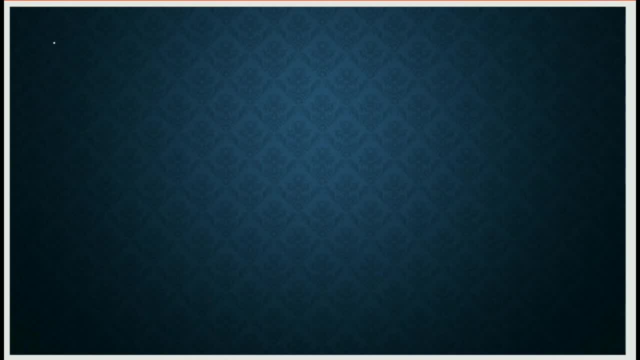 greater. So I will explain why this reverse order is coming. So there is two factors which depending upon the solubility. So what are the factors? lattice energy and hydration energy. So, for a salt, if lattice energy change, so there will be a change in lattice energy and hydration. 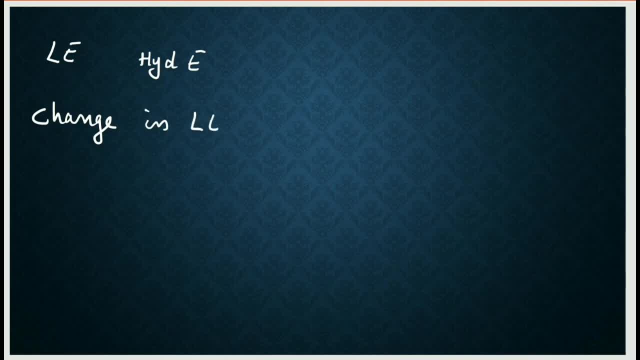 energy change. Change in lattice energy is greater. If the change in lattice energy is greater, then it's a major change in properties of the process. So that's why there is a reverse order and there is an exponential tendency to change in properties of the process. So when we talk about 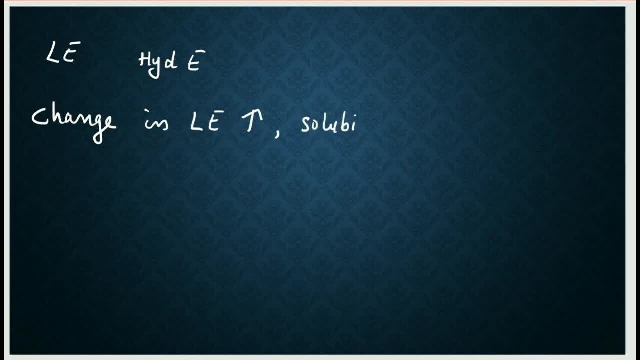 then solubility is increased. And if hydration energy is changed larger, then solubility decreased. So change in hydration energy increases, solubility decreases. So why fluorides and hydroxides have high solubility? Their lactose energy is increasing. So 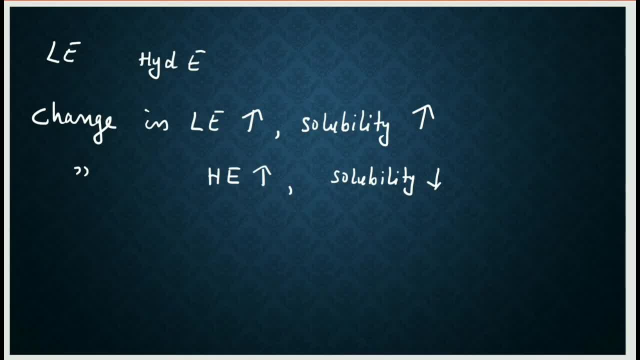 the solubility is increasing When lactose energy is increasing, solubility increasing And when hydration energy changes, increasing solubility decreasing And the lactose energy is depending upon the size. Lactose energy decreases when size increases. So beryllium. 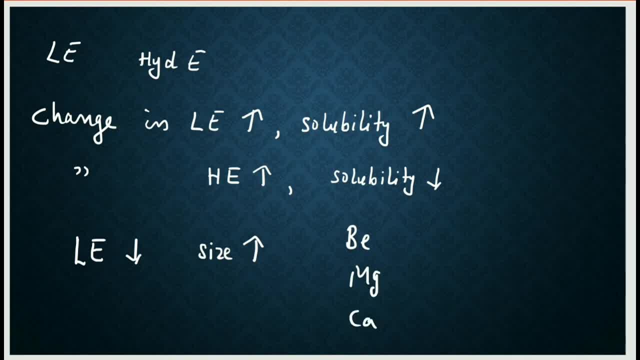 magnesium, calcium, So, which is having high size. Calcium is having high size, So lactose energy will be increasing. low lattice energy will be low. for calcium and for beryllium lattice energy is high because size is small. so lattice energy, similarly like ionization enthalpy, it is directly proportional. 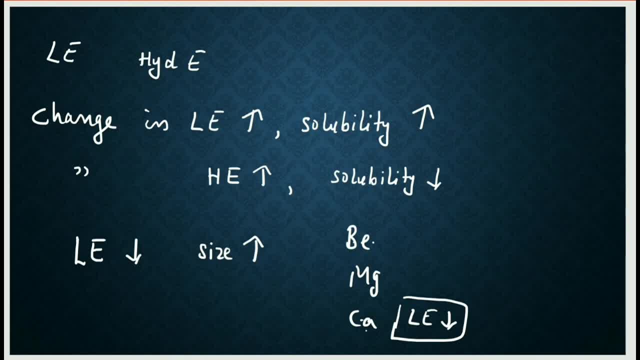 to or inversely proportional to size, directly proportional to one by size most compounds. on descending the group, the hydration energy decreases more rapidly than lattice energy. so when you move down the group, down the group that is from beryllium, magnesium, calcium, strontium and barium, down the group, the hydration energy changes decrease hydration energy changes. 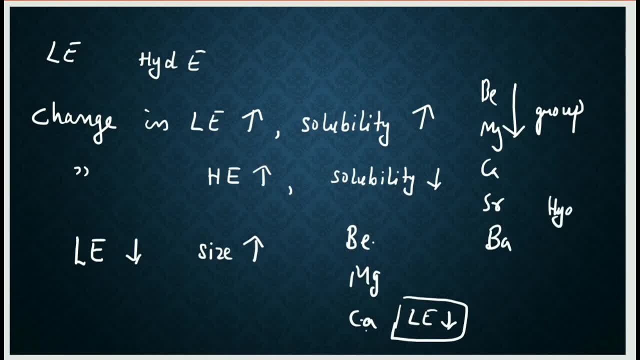 increased. so the hydration energy change is coming into main role. so what happened? the solubility decreases. when hydration energy changes increased, the solubility decreased. So for beryllium, magnesium, calcium, strontium, barium, the barium is insoluble, but 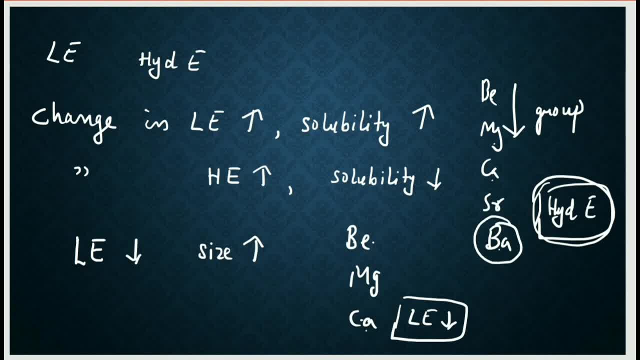 coming to fluoride and hydroxide, the compounds of barium hydroxide, barium fluoride or strontium fluoride. the hydration, not hydration energy, the lattice energy is coming into play. So when lattice energy is changing, the solubility is increased. So there is an exceptional case for fluorides and 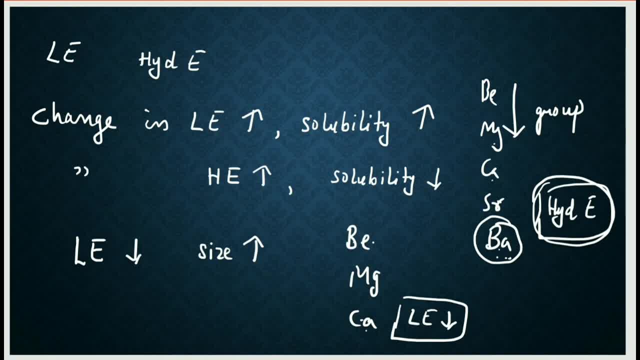 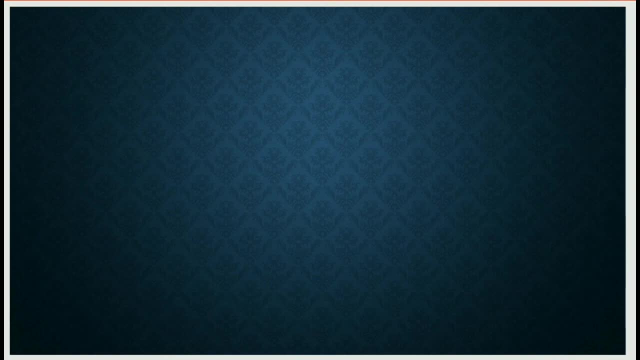 hydroxides the solubility increases when lattice energy change increases and for other salt the solubility is decreased only because the hydration energy change. Now we can discuss the compounds formed by alkaline earth metals. that is first one hydroxide, So calcium hydroxide is formed. 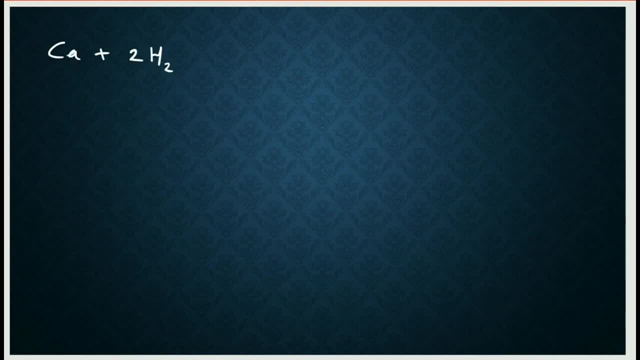 when calcium plus water is reacted, calcium hydroxide is formed. Similarly, all other hydroxide can be formed when calcium hydroxide is formed. So calcium hydroxide is formed when calcium is formed while reacting with the water. So when calcium is reacted with water, calcium hydroxide and 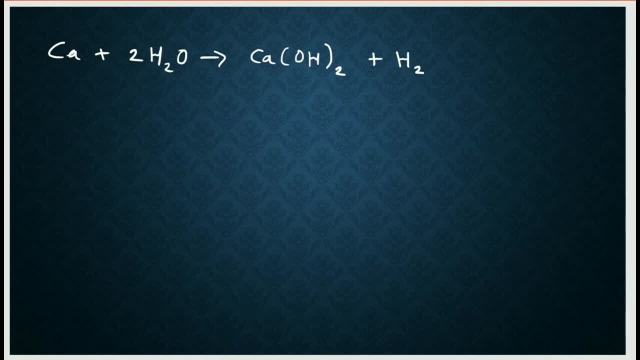 hydrogen gases evolved. And next one is beryllium plus NaOH Beryllium. one more thing. beryllium is an exceptional case in this alkaline earth metals like lithium. So in group 1, lithium was an exceptional case. In group 2, beryllium is an exceptional case. 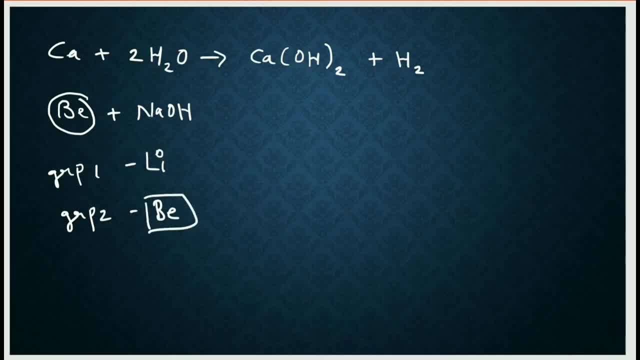 In many properties beryllium stand out. Beryllium have anomalous properties, So here beryllium plus sodium hydroxide will give a hydroxide, beryllium hydroxide, that is, Na2, beryllium hydroxide, BOH. 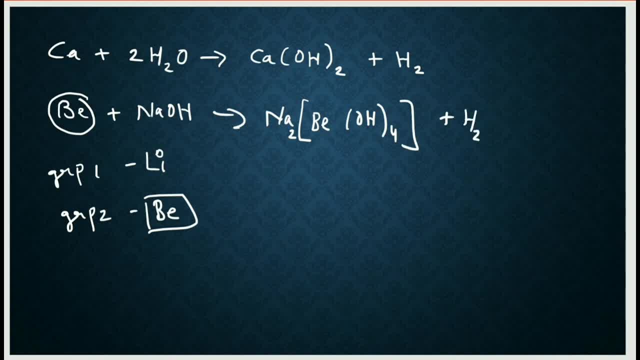 four times plus H2.. So this is a amphoteric hydroxide. amphoteric And all other hydroxides are basic. All other hydroxides of calcium strontium, magnesium, etc. are basic, But beryllium hydroxide. 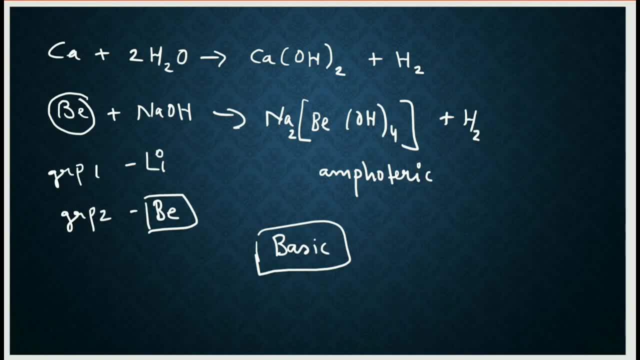 is amphoteric. And next compound is oxide, normal oxide. So in group 1 elements we discussed the normal oxide, monoxide, superoxide etc. Now in alkaline earth metal normal oxides are formed. How this is formed? A metal, alkaline earth metal, to metal, beryllium. So this is 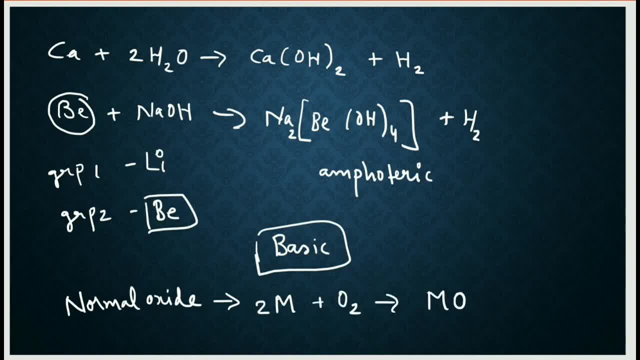 a normal oxide. This is a beryllium hvis focus the number of bars is. Graphite is dialy tay steht its necessity: 11.3, 50ca, 00 وس, 00, 12 C, 21.4, 15.8, 15.8, 16.6, 14.3, 15.4, 17.8, 21. 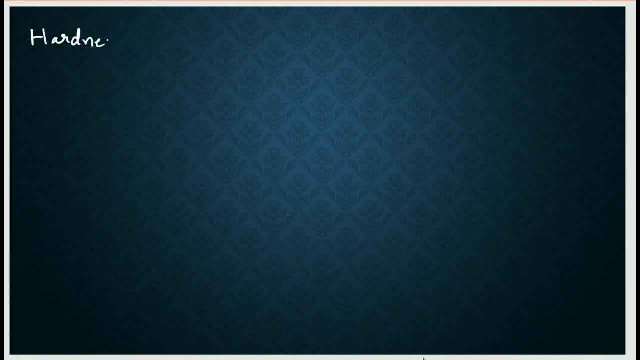 2 x 8: 16.5 water hardness of water. so what is hardness of water? there are two types of hardness: temporary hardness and permanent hardness. so the factor which affecting temporary hardness is what? magnesium bicarbonate. so temporary hardness is due to magnesium bicarbonate, bicarbonate, hco3, twice. 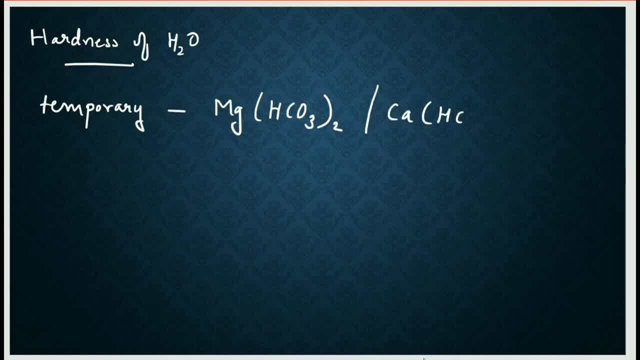 or calcium bicarbonate. so both are responsible for the hardness of water: magnesium and calcium ion. so magnesium bicarbonate is the reason for temporary hardness. and what is temporary hardness? it can be removed by boiling the water. so when you boil the water, the temporary hardness- magnesium bicarbonate- can be removed. and permanent hardness? hardness means permanent hardness. 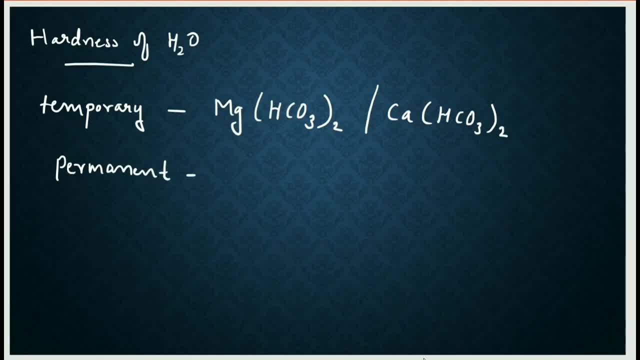 so permanent hardness cannot be removed by boiling the water. So permanent hardness is due to magnesium sulfate or calcium sulfate. So sulfate of magnesium and calcium is responsible for permanent hardness. Then, talking about the sulfates of alkaline earth metals, beryllium sulfate and magnesium sulfate are soluble. Beryllium sulfate and magnesium sulfate. 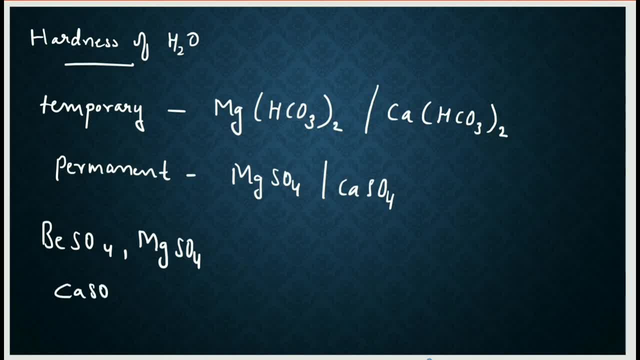 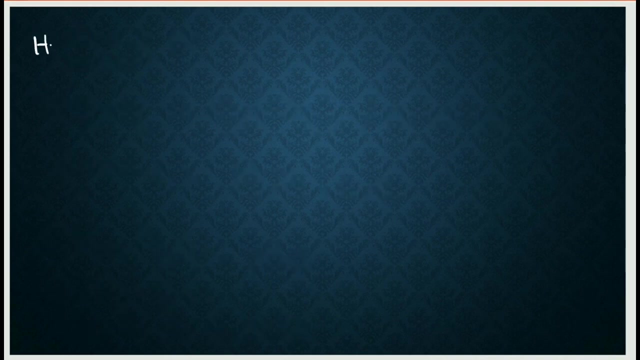 are soluble and calcium sulfate is sparingly soluble, and strontium, barium, radium are insoluble. So calcium sulfate is sparingly soluble and beryllium sulfate and magnesium sulfate is soluble, and strontium, barium, radium sulfate are insoluble. Type of compounds are: 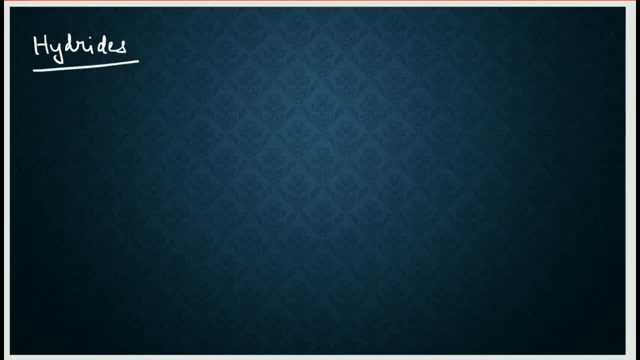 hydrides. So the general formula for hydrides is MH2.. How the hydrides are formed? The metals are reacted with H2. So you will get MH2, that is, hybrid, And BEH2,. beryllium hydride is difficult to prepare and it is less stable, So beryllium 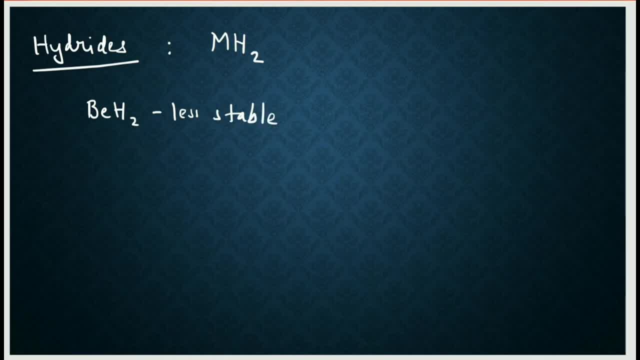 hydride is difficult to prepare And how this can be prepared. 2 BECL2, beryllium chloride is taken and it is reduced with lithium aluminium hydride. When you reduce lithium aluminium hydride, when you reduce beryllium chloride with lithium aluminium, 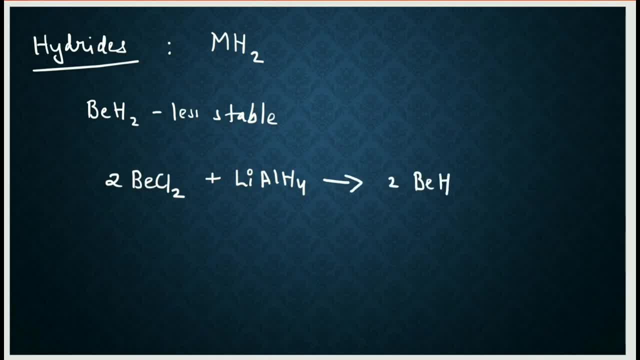 hydride, you will get 2 BEH2, beryllium hydride plus lithium chloride plus AlCl3.. So this is the reaction. Just remember this reaction: Beryllium hydride is obtained by reducing beryllium chloride. 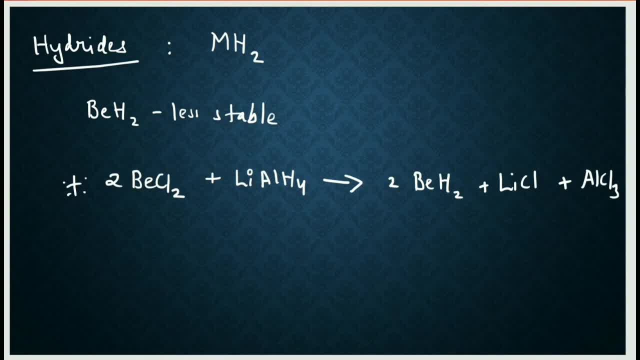 with lithium, aluminium hydride And calcium hydride. strontium hydride, CaH2, beryllium hydride are formed when heating with hydrogen and they are ionic. They are ionic compounds And Beryllium hydride, BEH2, and magnesium hydride, MgH2, are covalent, So the difference is. 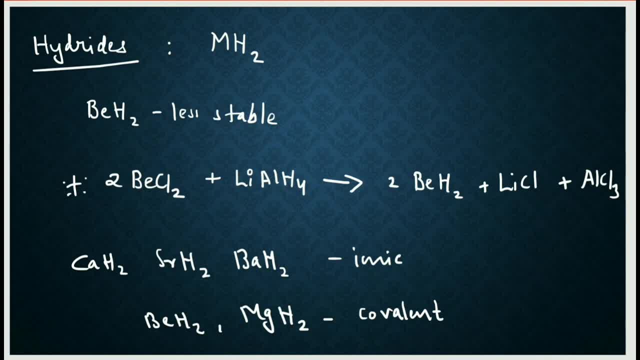 calcium strontium, beryllium hydrides are ionic, which contain H minus ion, So that is ionic, And beryllium and magnesium are covalent. So this is the reaction. So this is the reaction And 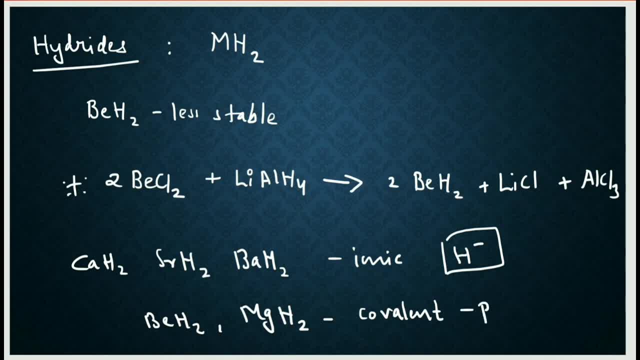 covalent and they can be in polymeric structure. So they can be polymeric structure. Polymeric structure means BEH2, can be in polymeric structure means BEH2N times. So 3 sender 2 electron bonds are present. What is 3 sender 2 electron bonds? The banana bonds, The banana bonds which is seen. 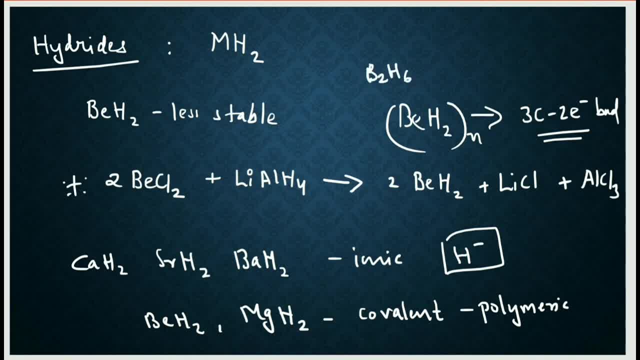 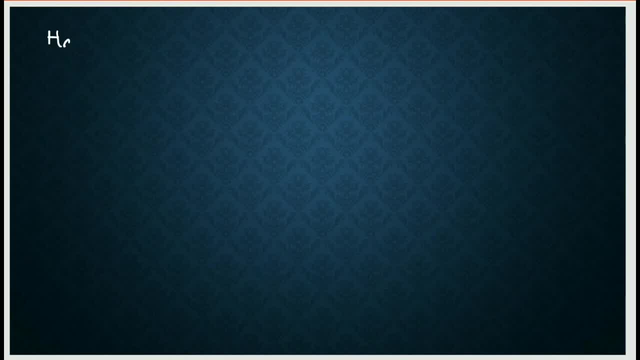 in boranes. So when you analyze the structure of borane you can see a banana bond. Next is halide. So alkaline earth metal can form halide also. The general formula is MX2.. So X means a. halide- any type of halide- chlorine, bromine, iodine, M is metal and it is formed by heating metals with halogen. So anhydrous halides are polymeric. What is anhydrous halides? 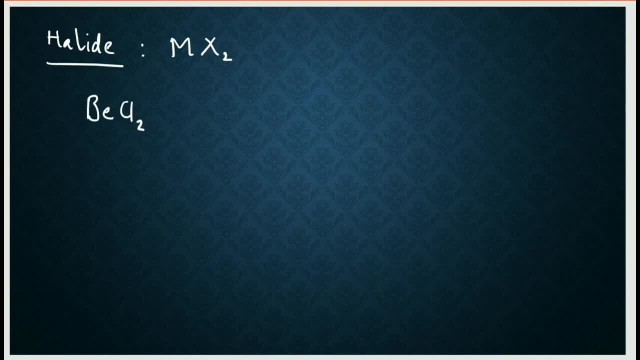 Halide of beryllium, BECl2.. So BECl2 is anhydrous halide and it can be in polymeric structure, that is BECl2 twice. So I already said polymeric structure can contain 3 sender, 2 electron bond. 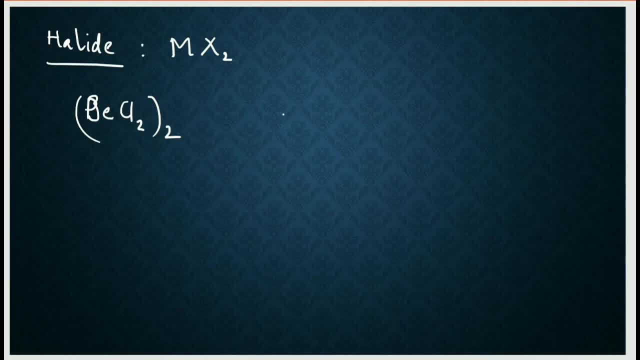 Then chloride bromide, iodide of magnesium, calcium, strontium, barium are ionic. So magnesium, calcium, strontium and barium chloride and iodide bromide are ionic. These are ionic and they are lower melting point and boiling point. They have lower melting. 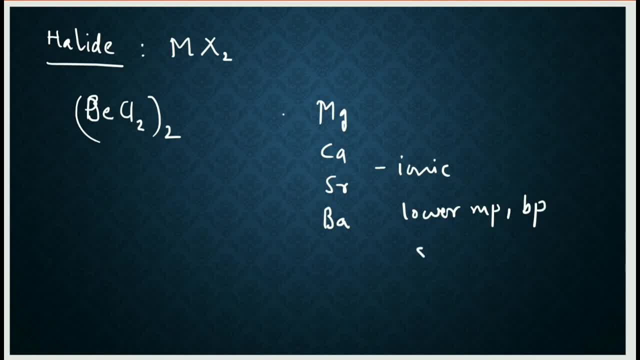 point and boiling point. and these are soluble in water. So these are soluble in water also: Magnesium iodide or chloride, etc. And next one is nitride. So nitride, the general formula is what- M3N2 for nitride. 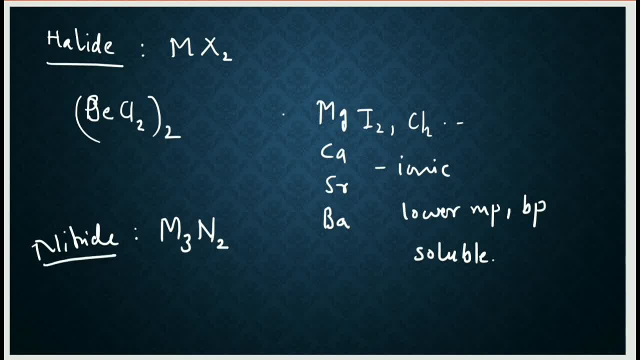 The M3N2 is formed, how The metal is reacted with dinitrogen. M plus N2 will give M3N2 nitride. And one more thing: BE3N2, beryllium nitride is a volatile, So beryllium nitride is a volatile. 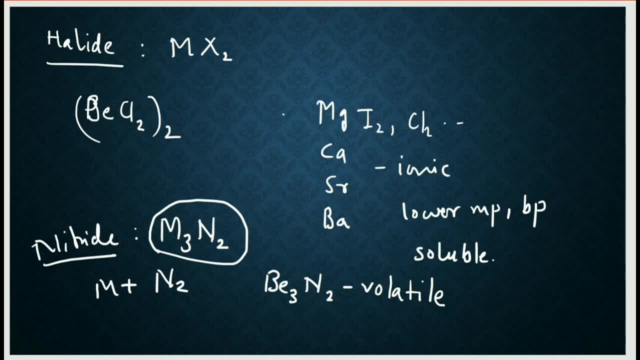 and others are non-volatile. Others means magnesium, calcium, strontium, barium nitrides- are non-volatile. So beryllium nitride is volatile. So beryllium nitride is volatile. So beryllium nitride is volatile. 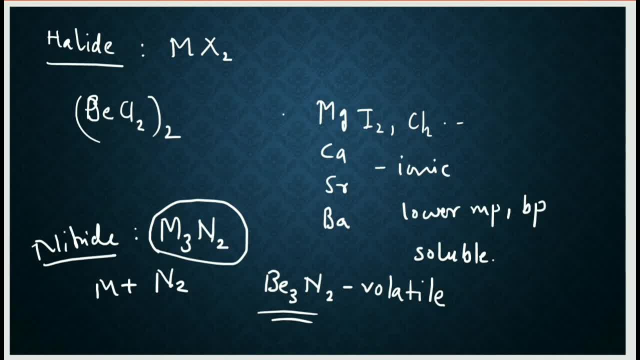 So I already said beryllium have different properties. It stand out in the alkaline earth metals And calcium nitride, Ca3N2,. calcium nitride is formed and calcium nitride is reacted with water- H2O- you will get calcium hydroxide. So when calcium nitride is reacted with water, 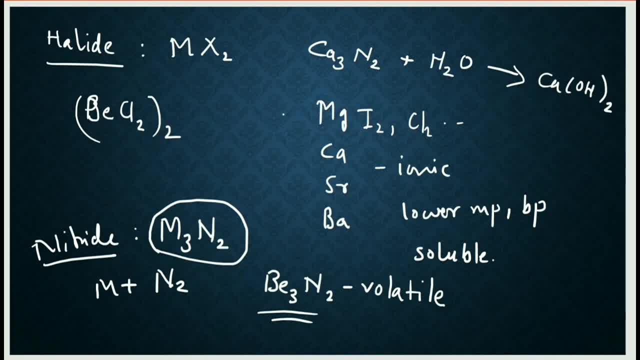 you will get calcium hydroxide. So there are chances to ask these reactions. So in one question one year, a question was asked about the group 1 metals, How the oxides are formed with lithium, So how the oxide is formed. Li plus O2 will give LiO, that is a oxide. So similarly, 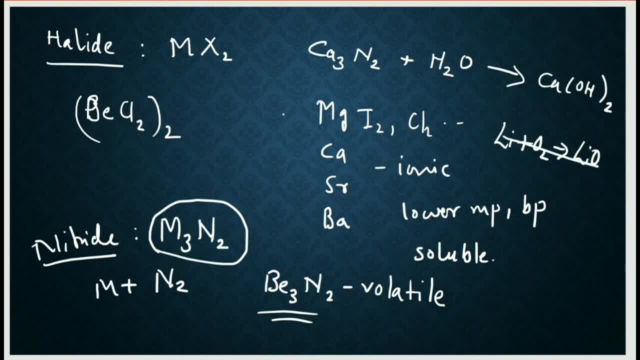 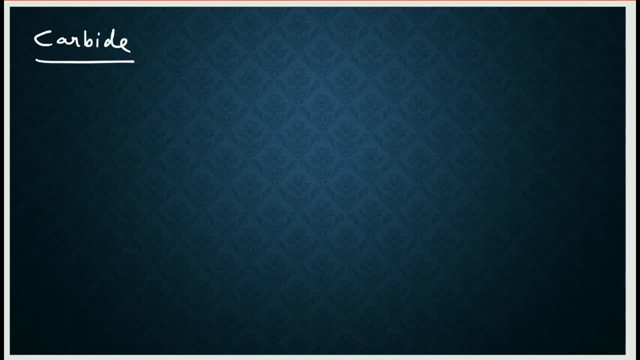 these type of reactions can be asked as question. Next class of compound is carbide. So what is the formula for carbide? MC? So carbide is a compound that is formed with lithium, So carbide is formed with lithium. So carbide means Be2C, Be2C- beryllium carbide is a brick red colored carbide. 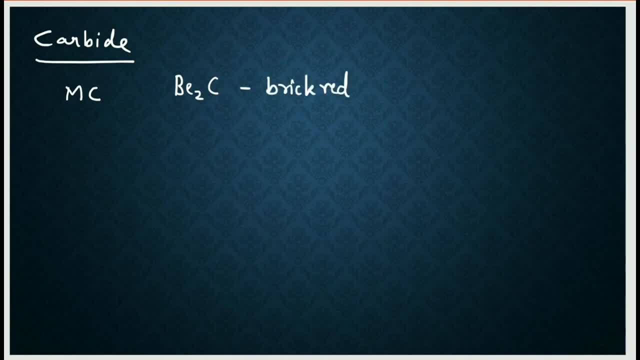 Brick red color carbide. And BeO- beryllium oxide, is heated with carbon to form Be2C- beryllium carbide. So BeO is heated with carbon to form beryllium carbide and it is a ionic carbide. It is a ionic. 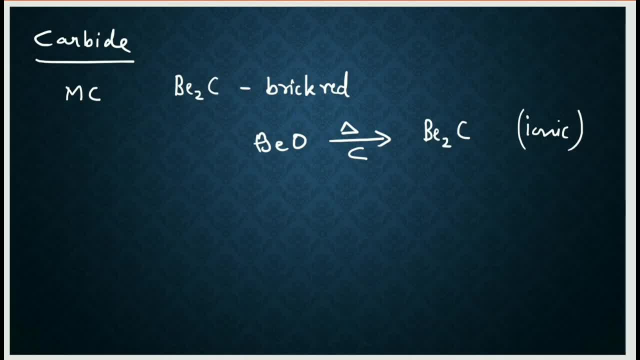 carbide And magnesium, calcium, strontium, barium form carbides of formula MC2.. So in beryllium carbide the formula is Be2C, that is M2C, And for other magnesium, calcium, strontium and barium. 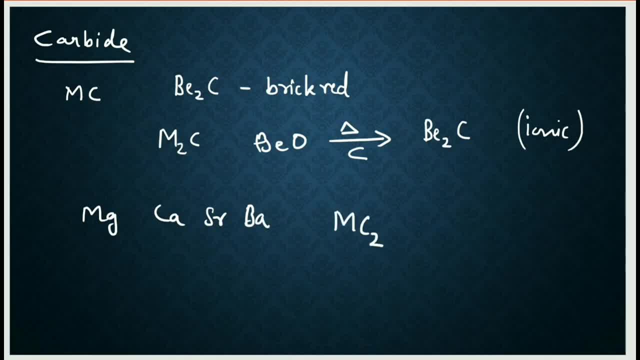 the carbide formula is MC2.. So that means MGC2, not Be2C, not MG2C, It is MC2.. So that is the beryllium. In beryllium the carbide formula is BE2C, And in magnesium, calcium, strontium. 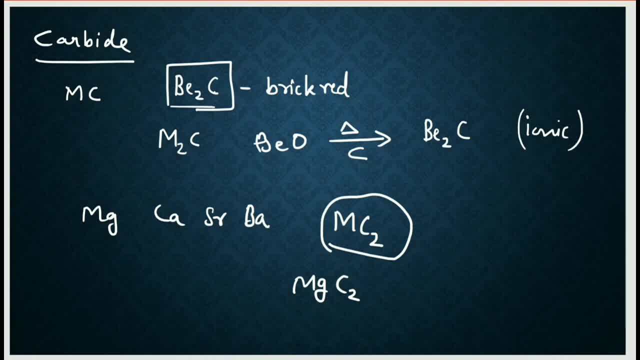 barium radium. MC2 is the formula of carbide, And another important point to remember is calcium carbide. So what is the formula of calcium carbide? MC2, that means CaC2.. CaC2, calcium carbide is heated with nitrogen. So what happens? CaC2 plus N2 will form. 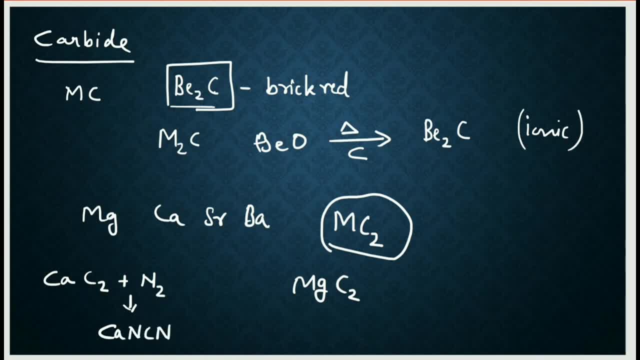 Ca N C N, Ca N C N plus C, So Ca N C N is what Calcium cyanamide, So cyanamide cyanamide is formed. Cyanamide means N, double bond, C, double bond, N, 2 minus Cyanamide ion is. 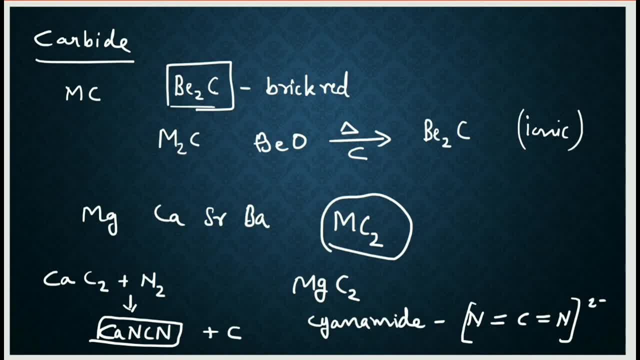 formed N double bond, C double bond, N 2 minus, And it is isoelectronic with carbon dioxide. So this has C, So it has the same electrons as carbon dioxide, So it is isoelectronic, So there is a chance to. 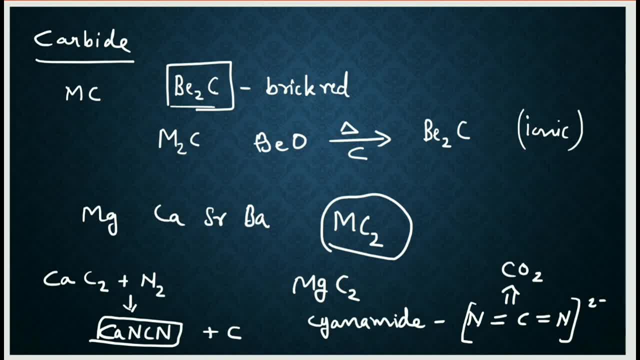 ask: cyanamide is isoelectronic with CO2.. And when barium nitride, that is BA, sorry, barium carbide, BAC2.. When barium carbide is reacted with N2, there is not forming cyanamide. But 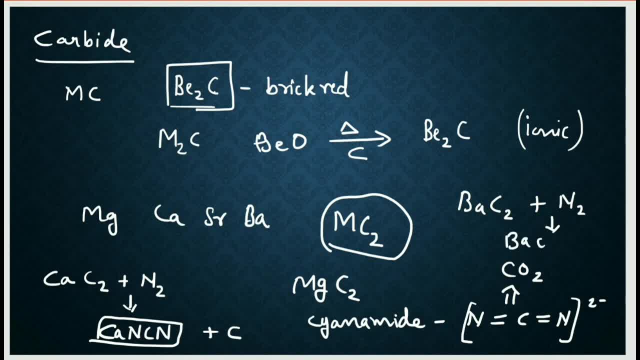 instead of cyanamide. what is forming BACN2.. Cyanamide- BACN2- is formed when barium carbide is reacted with dinitrogen, So carbide's formula is M2C. M2C for beryllium and MC2 for other MGs: calcium, strontium, barium, etc. 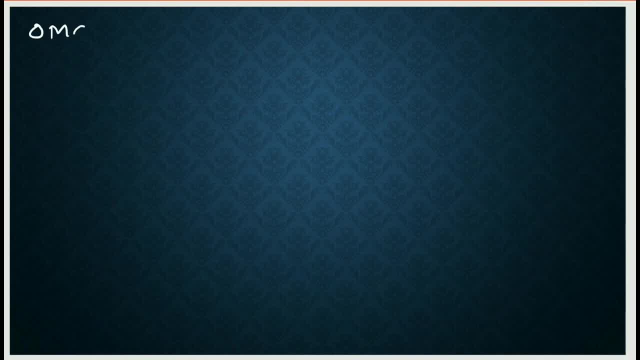 Now coming to organometallic compounds formed by alkali metal organometallic compounds. So the important organometallic compound is Grignard reagent. So the general formula of Grignard reagent, how to prepare. 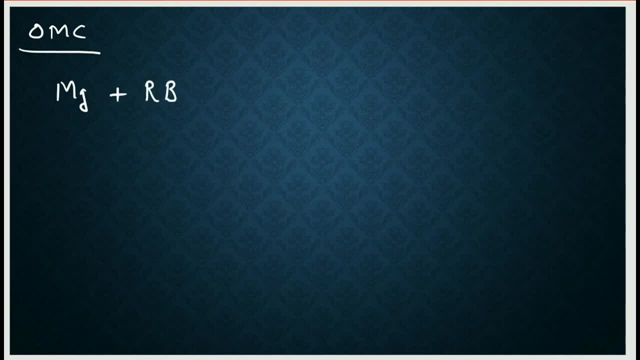 Magnesium plus RBR. R can be alkyl or aryl group in presence of either Dry either Dry either. So in presence of dry either, magnesium plus RBR is heated. So what happened? RMGBR? So this is Grignard reagent, RMGBR. 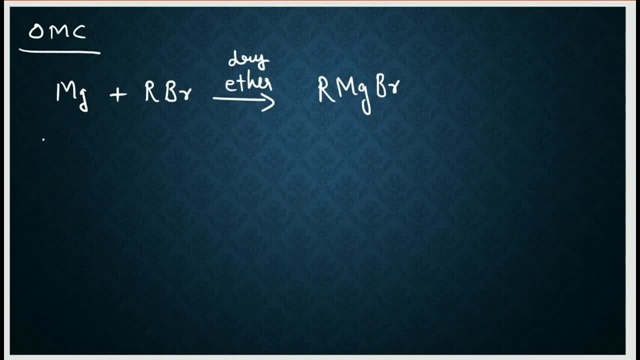 And one important point is iodides are most reacting Iodide. So in instead of bromine. if iodide is there it is highly reactive And chlorine is least reacting. And alkyl: if R is alkyl then it is highly reactive than aryl. 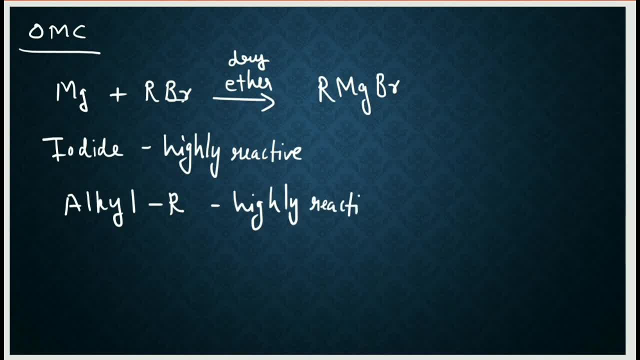 Highly reactive. So if R is alkyl then it is highly reactive than aryl group. So R should be alkyl group. and if instead of bromine you can take iodine, also it will be highly reactive. So the reactions of Grignard reagents are 2RMgBr plus water. 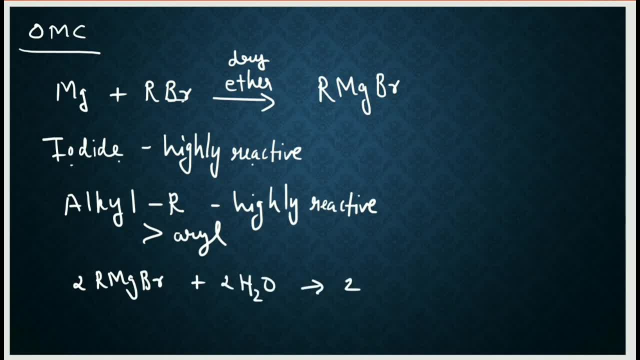 So what you will get 2RH, a hydrocarbon plus magnesium hydroxide, MgOH2 plus magnesium bromide MgBr2.. So a hydrocarbon is formed when Grignard reagent is reacted with water. So that's one reaction and so many reactions are there with Grignard reagent. when Grignard 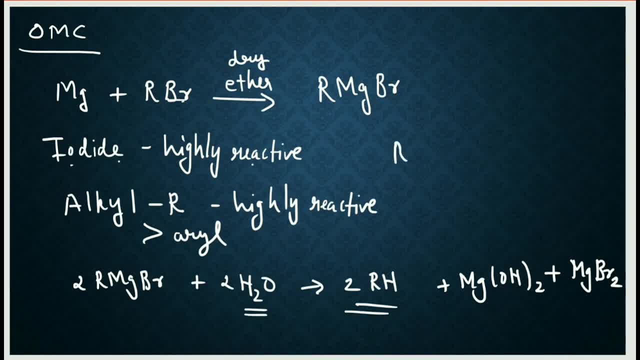 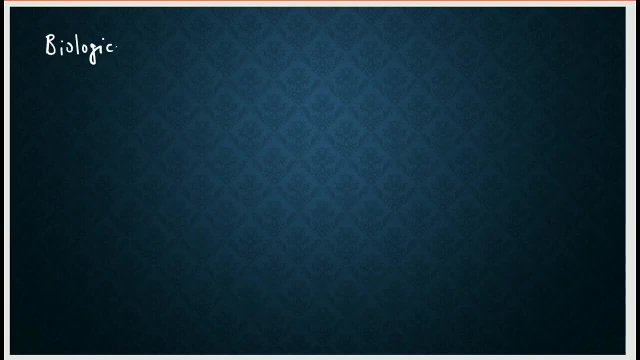 reagent is treated with carbon dioxide. So RMgBr plus MgCO2 in presence of a acid, what you will get? a carboxylic acid, RCOH. Moving on to biological importance, So biological importance of alkaline earth matters, that is. 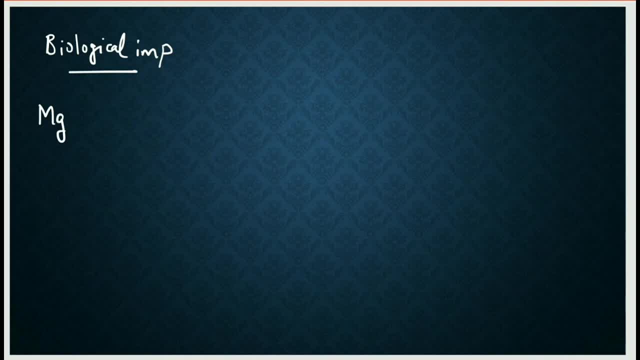 mainly magnesium and calcium. So we will talk about magnesium 2 plus and calcium 2 plus biological importance. So magnesium 2 plus is present in animal cell. It is present in animal cells and calcium 2 plus is present in animal cells. So magnesium 2 plus is present in animal. 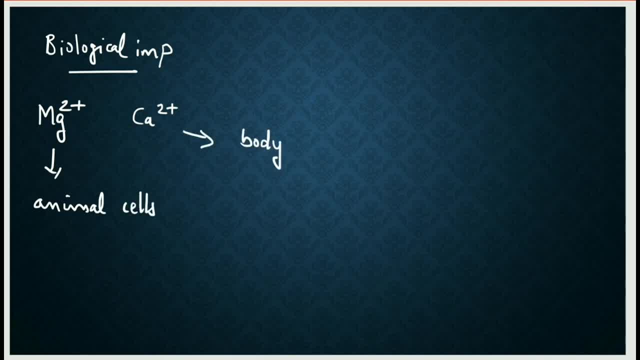 cells and calcium 2 plus is seen in body fluid, So it is outside the cell body fluid. So it is same like the sodium and potassium, Sodium and potassium salt. Sodium and potassium salt Same like sodium and potassium salt. that is the concentration in outside and inside cells. So 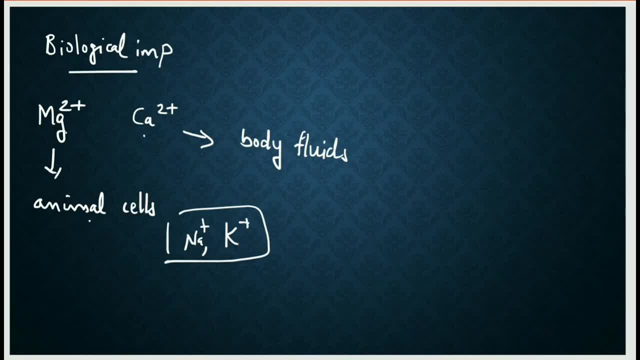 magnesium is inside animal cells and calcium is inside body fluid that is outside the cells, And magnesium 2 plus. the major complex formed by magnesium 2 plus is chlorophyll, So it is the main important complex. Chlorophyll contains magnesium 2 plus And calcium 2 plus is present in bonds. Should be present. 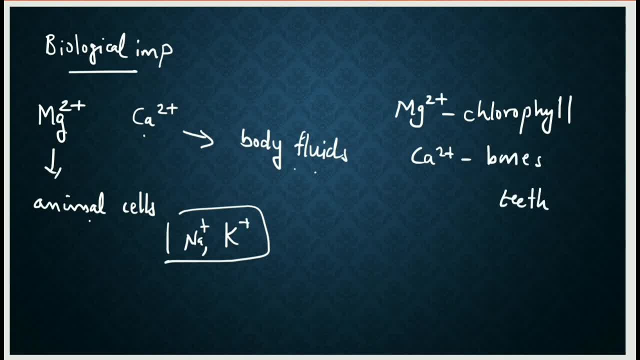 in bonds, teeth etc. So in bonds and teeth calcium 2 plus is present and in teeth it is formed in a patchite that is the formula CA3PO4 twice, Ca3 po4 twice, And in enamel on teeth. enamel on teeth it is fluorapatite. Another uses of calcium 2 plus is it is important for 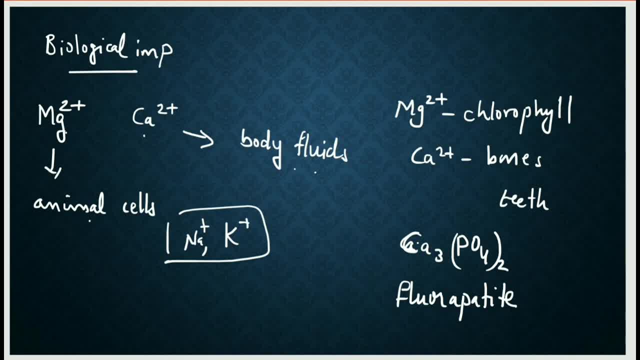 blood clotting and required to trigger contraction of muscles. So for contraction of muscles the calcium 2 plus is required, mainly regular beating of heart. So beating of heart to trigger contraction of muscles. for blood clotting calcium 2 plus plays an important role. So the biologically 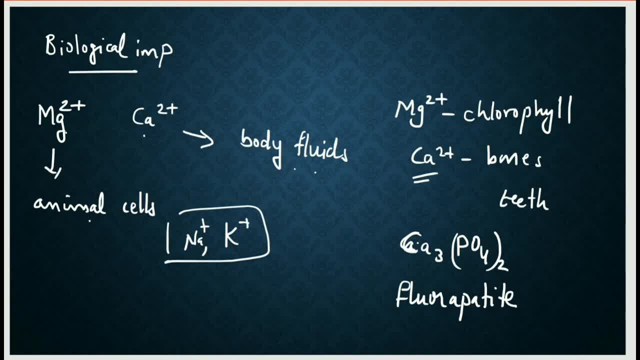 importance of magnesium and calcium is what magnesium is present in chlorophyll and it is in animal cells. Calcium is in body fluid and it helps the strength of bones, teeth, the enamel of teeth and it is fluorapatite in enamel of teeth.